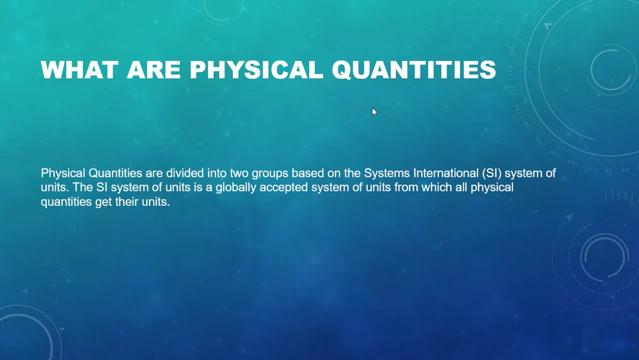 The SI System of Units is a globally accepted system of units from which all physical quantities get their units. Now, physical quantities are are divided into base quantities and derived quantities, And we'll be looking further at these two types of quantities: base quantities and derived quantities. 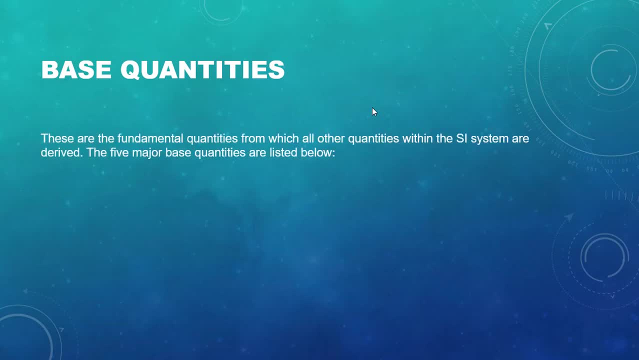 So, first of all, base quantities, right, these are as the name suggests. these are fundamental quantities from which all other quantities within the SI System are derived, And the SI System of Units actually assigned seven base quantities. right, but for your level, we consider the first five, and they are listed below. 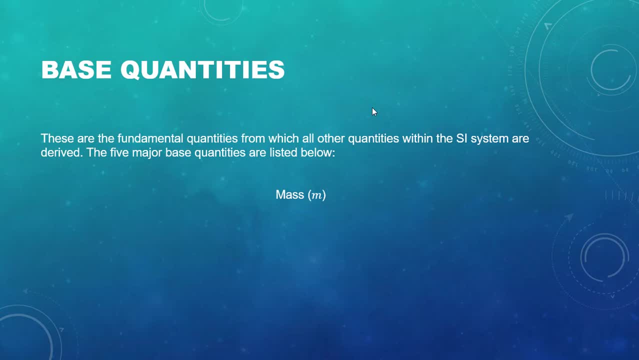 So the first one is mass, and its symbol is a lowercase m. We have length, and its symbol is a lowercase l. We have time, its symbol is a lowercase t. We have electric current, and its symbol is a capital I. And we also have temperature, and the symbol for temperature is a capital T. 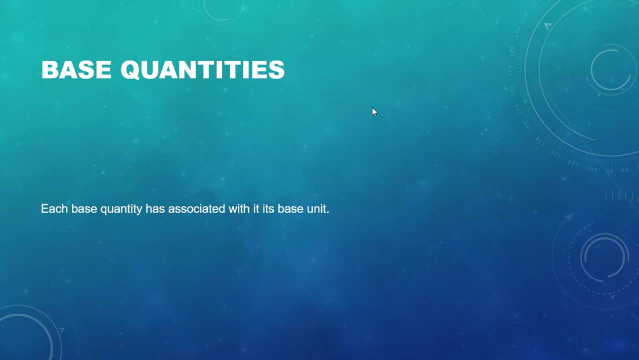 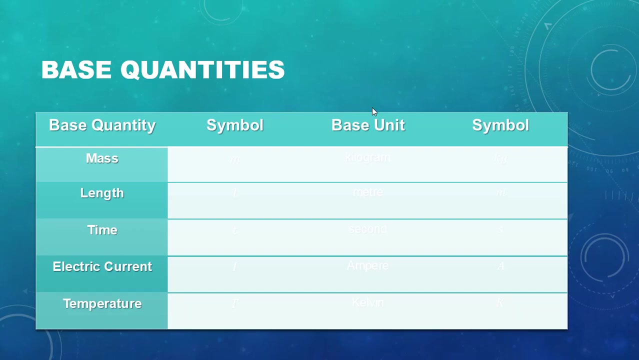 Now, each base quantity has associated with it a base unit. So in the case of mass, which is our physical quantity, specifically a base quantity, we have a base unit. The unit of mass, or the associated unit of mass is the kilogram. So we're going to look at those shortly. So here we have our table with the five base quantities: mass, length, time, electric current and temperature. 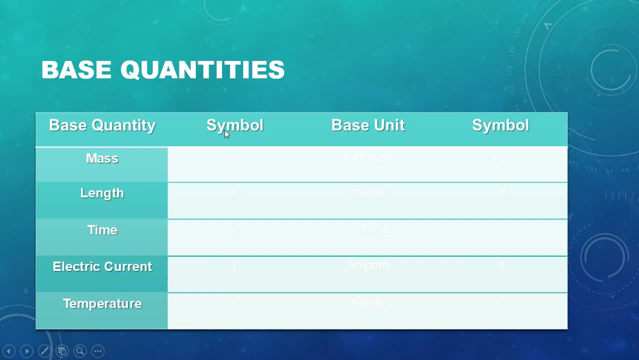 All right, then we're going to look at the symbol of each base quantity, the base unit of each base quantity and the symbol of each base unit. So, for mass, the symbol of mass is lowercase m, as we have seen before. Its base unit is the kilogram and the symbol is kg. 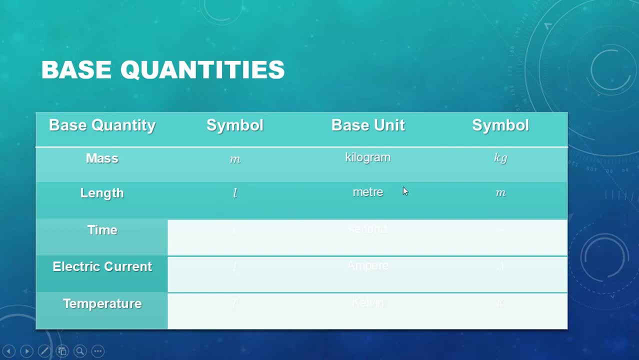 For length symbol again is l- Base unit meter, and the symbol for the base unit is m. Now I usually see where students would confuse the symbol for the base unit for the base quantity. both of them, as you can see, are separate. so, for example, 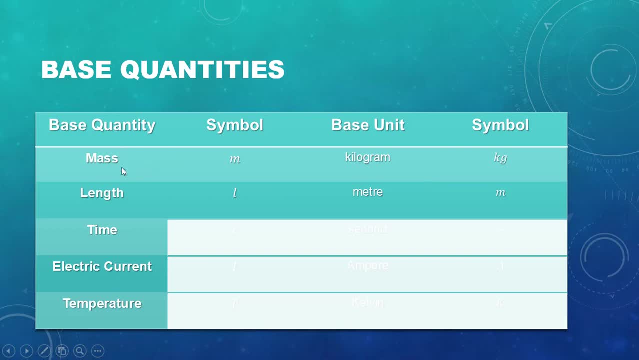 again, in the case of mass, the symbol for the base quantity mass is M and the symbol for the base unit of mass is kilogram, which is kg. right, so you have to be aware of that so you can actually make that differentiation. then time: the symbol for time, the quantity time is T. the unit base unit for time is the. 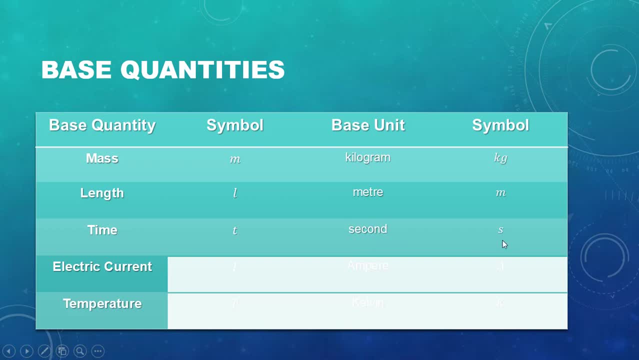 second, and that symbol is a lowercase s. similarly, for electric current we have a capital I, base unit, ampere, and its symbol is an A. then for temperature, symbol T, base quantity, Kelvin, and its symbol is a capital K. so this table here will become very critical when we go further. so if you want to take a minute and actually 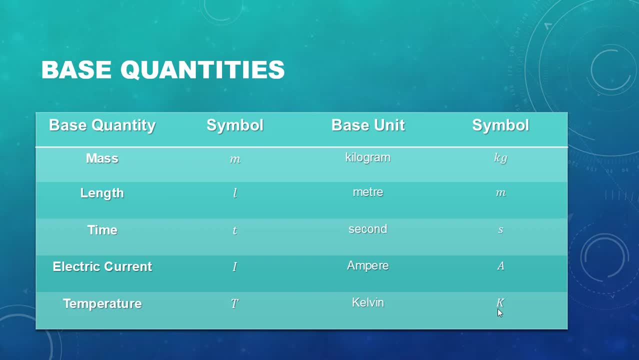 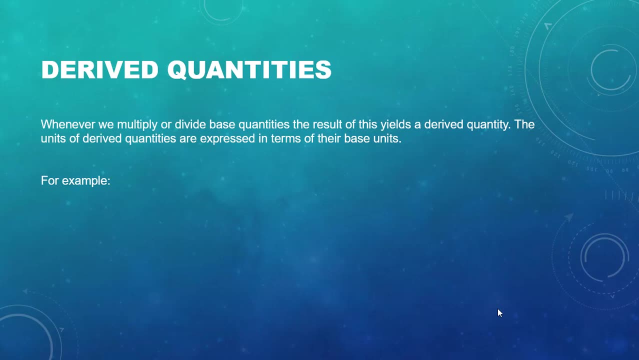 write this table down. I would advise you do so. so let's now look at derived quantities. so we're saying now, whenever we multiply or divide base quantities, the results of this yields a derived quantity, right? so basically, our derived quantities are formed from base quantities and again base quantities. 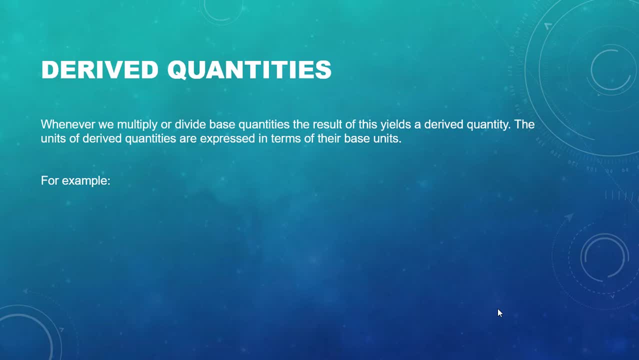 are the basic, are the fundamental quantities from which all other quantities are derived. so we get base quantities when we, whenever we multiply or divide our fundamental quantities. now the units of derived quantities are expressed in terms of their base units. so, for example, we have area which is our. 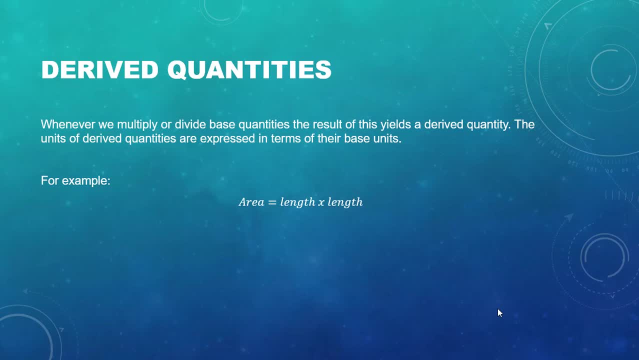 derived quantity and that is found by multiplying the length of an object times its length. so if we were to express some- the units or the base unit of length are expressed here in terms of its base unit, we can see where we'll get our derived unit. so here again is length times length the base quantity. 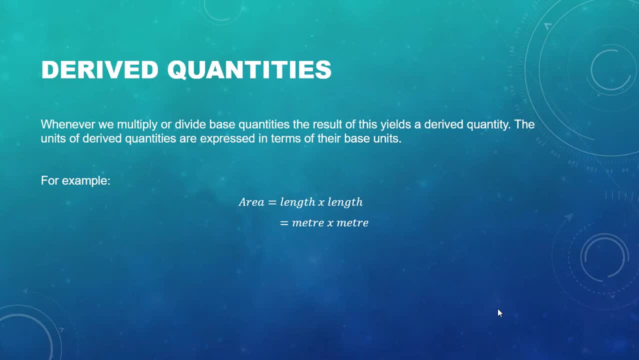 for length at the base unit for the base quantity length is meter and that is the base unit of length, or the base unit for the base quantity length is meter. right and I'm. its symbol is a low case M, so we write meters, times meters, and we 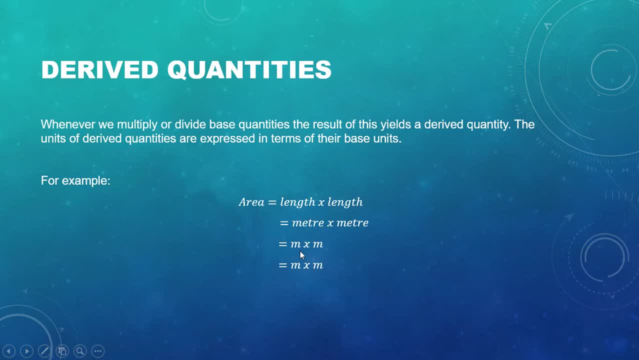 write it as in a symbol form: M times M right. and then if we multiply M times M, we get M squared. so the unit, the SI unit for area, therefore, the SI unit for the derived quantity area, therefore, is the meters squared or the square meter right. here's another example: speed is defined as the distance moved over a. 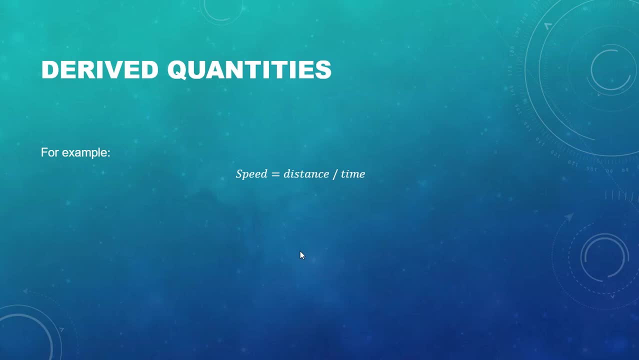 particular time. so we write that some distance divided by time know the. because distance is a length, the base unit of distance is the meter and the base is the distance, and the base unit of distance is the meter and the base unit for time is the second. so we write: meters divided by a second, alright, and 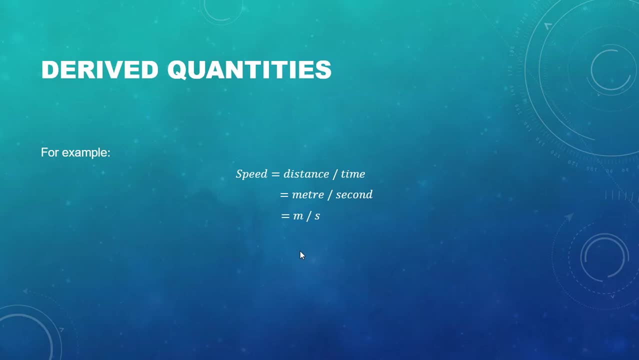 the right in symbol form, right M and s, and then we get that our derived unit for speed, which is a derived quantity, is meters per second. alright, and we can express them as in this form, or we can express it on with an exponent on the seconds, and this exponent time simply means that 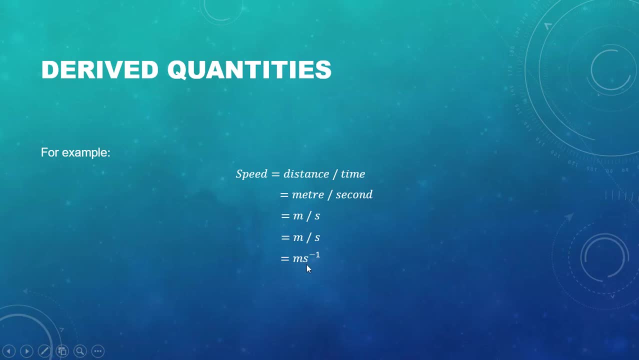 seconds is in the denominator. Okay, so let's continue with our look at derived quantities. So sometimes, when derived quantities are formed from the multiplication or division of base quantities, the results can be too complicated and therefore difficult to write. So to solve this, what we do, we give. 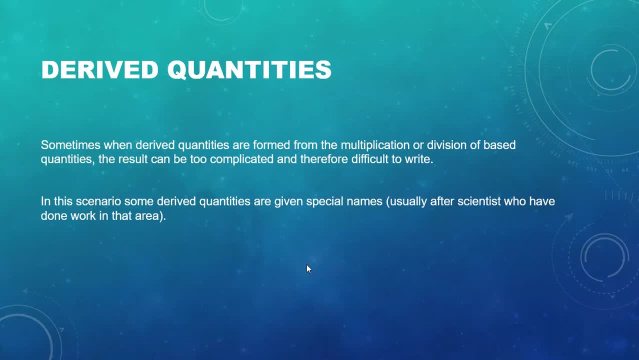 these derived quantities special names, and they are usually of the famous scientists who have done some work in that particular area. So, for example, the kilogram meters per second squared, which is basically mass multiplied by acceleration, is the SI unit of force. However, we give this: 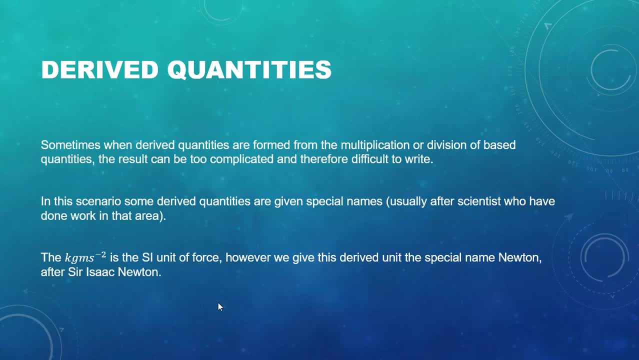 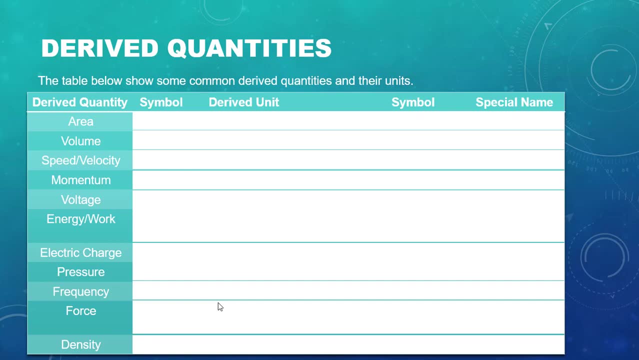 derived unit, a special name, Newton, after Sir Isaac Newton. Now here's a table of some common derived quantities and their units. So we have area, right, and its symbol is A, capital A, and the derived unit of area is the square meter and its symbol is: 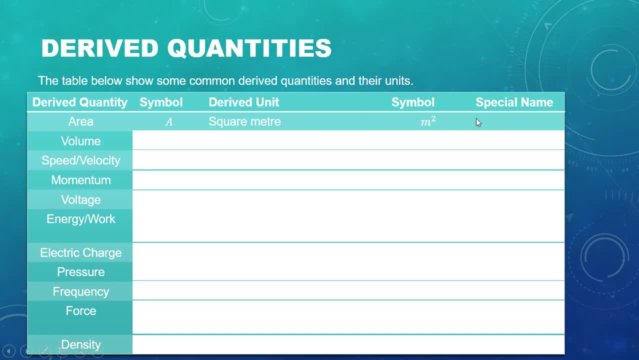 meters squared right, and this one doesn't have a special name because, as you can see, the unit is very easy for us to write. It's just meters with an index of 2.. Then we have volume. Its derived unit is the cubic meter and we write that as meters cubed. 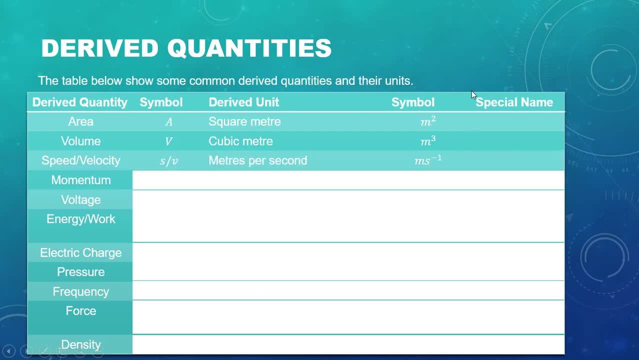 or m to the power 3.. Then we have speed or velocity. The symbol for speed is S and the symbol for velocity is V, And its derived unit is the meters per second, written as ms minus 1, or m slash s. whichever way is correct. 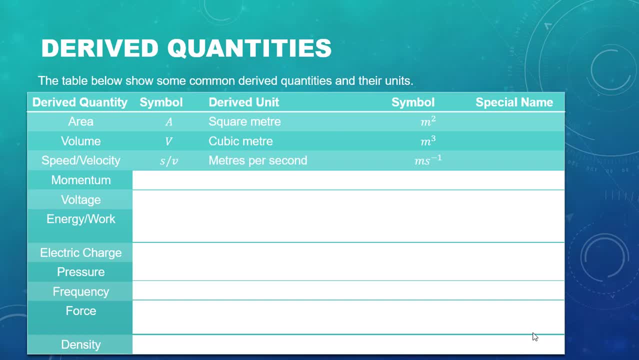 Okay, so the next one we look at is momentum. The symbol for momentum is P And its derived unit is the kilogram meters per second, written symbolically as kgms to the minus 1.. Our next derived quantity is the voltage. 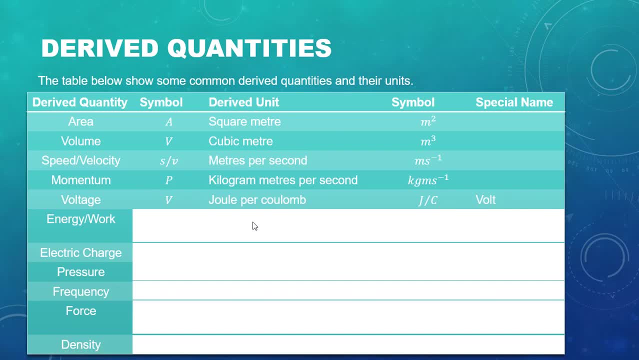 and its derived unit is the joule per coulomb, written as j divided by c or jc minus 1, and we give it the special name volt after the famous scientist Alexandra Volta. Derived quantity we look at is energy, which is energy at work. 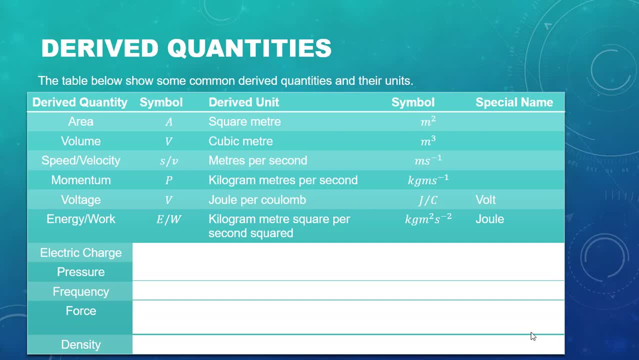 and that symbol is E or W energy, for E for energy and W for work, And that's a kilogram meter squared per second squared, and its symbol is kgms, squared times second per second squared. So it's kgm squared second minus 2, and we give it the special name joule. 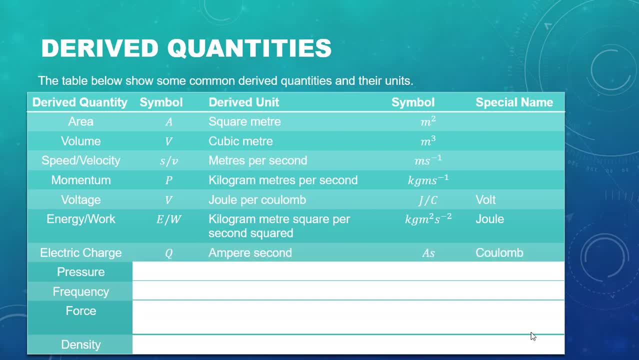 Next one we look at is the electric field. It's the electric charge, its symbol is C And we the derived unit is the ampere second, and the symbol is written as, As, and we give it the special name coulomb. 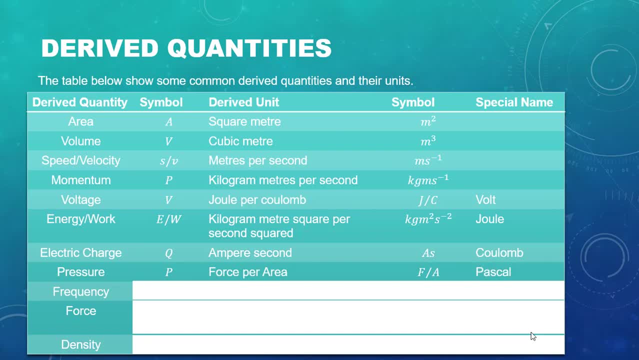 Next one we look at is pressure, which is force per unit air, and the symbol is F over A and we give it the special name pascal. Next one we look at is the frequency, which is F and the derived unit is per second. 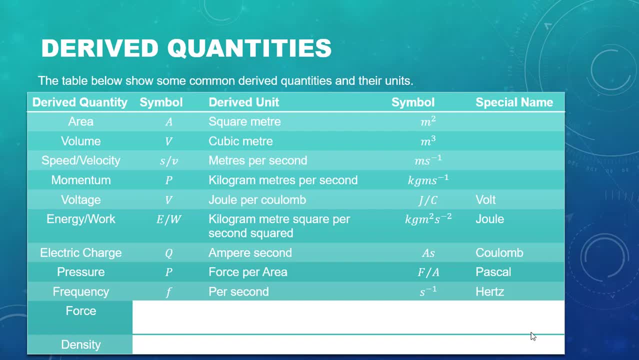 And we give it. it is written as S to the minus 1,, seconds to the minus 1, and we give it the special name hertz. Next one we look at is force. We talked about this one before. that's a capital F. 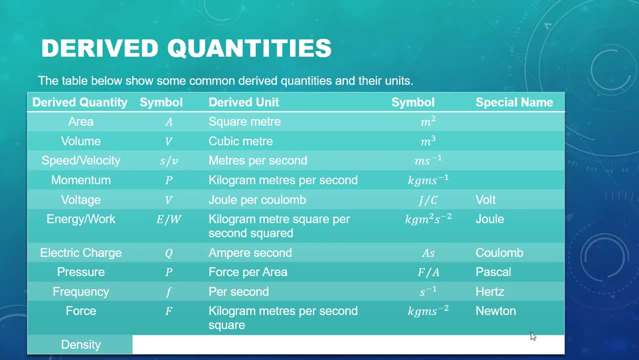 Kilogram meters per second squared, and it is written symbolically as kgms to the minus 2, and we give it the special name joule. Next one we look at is density, which is the kilogram per meter cube or kilogram per cubic meter, and we write it as kgm to the minus 3.. 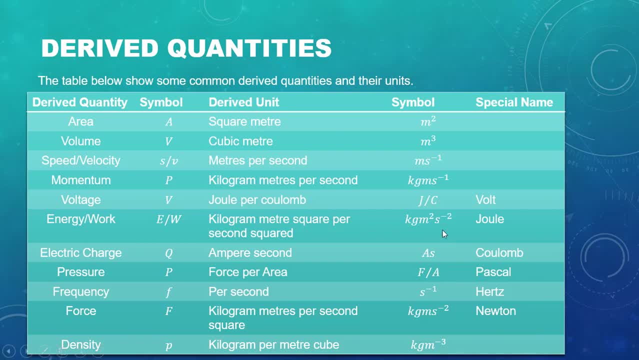 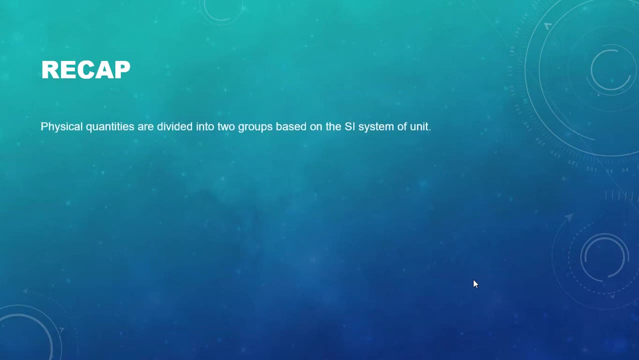 So this table here actually demonstrates some of the common physical quantities that are derived quantities and some of the quantities that are given special names. So in recapping we say that physical quantities are divided into two groups based on the SI system, And the SI system of units is a globally accepted system of units. 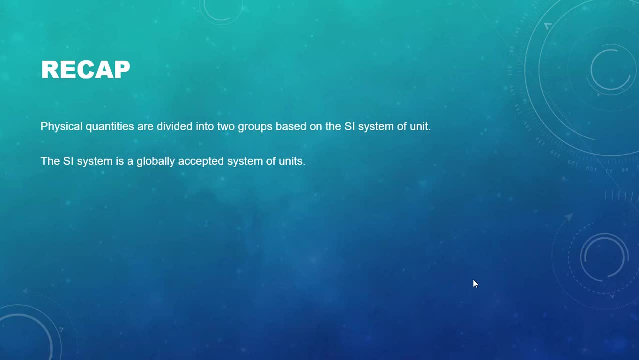 and we say that all physical quantities get the units from this system. Then there are five base quantities, namely mass, length, time, electric current and temperature. When we multiply or divide base quantities we get a derived quantity And some derived quantities can be complex to write. 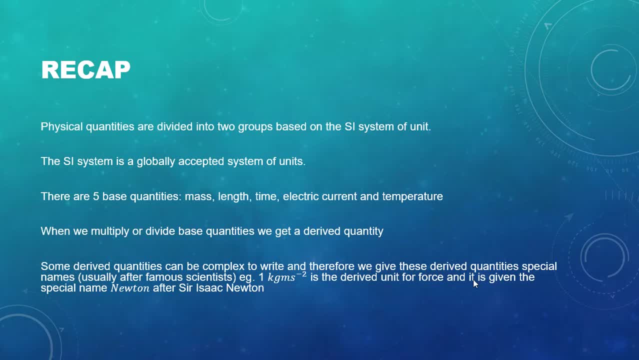 and we can write them special names, and this is usually after famous scientists, For example, the Newton, which is the kilogram meters per second squared, and it is named after Sir Isaac Newton. So this was our look at physical quantities. If you have any questions, please post them in the comments, send me an email.